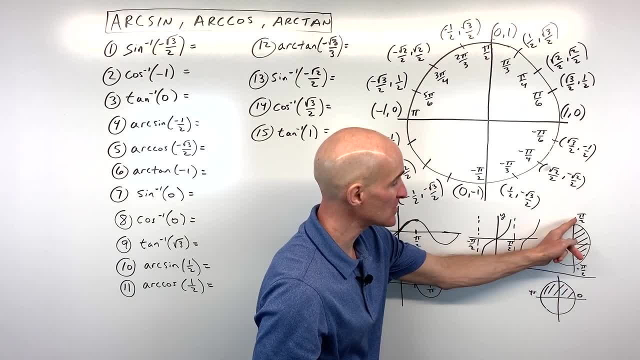 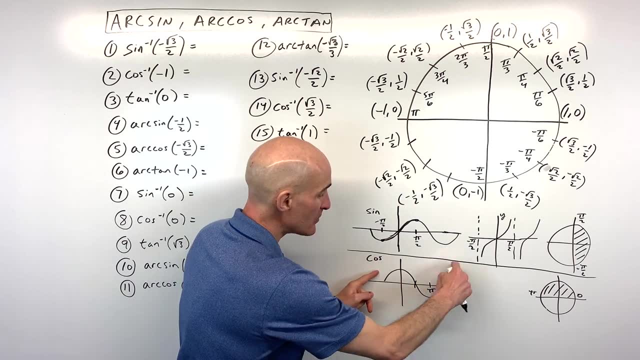 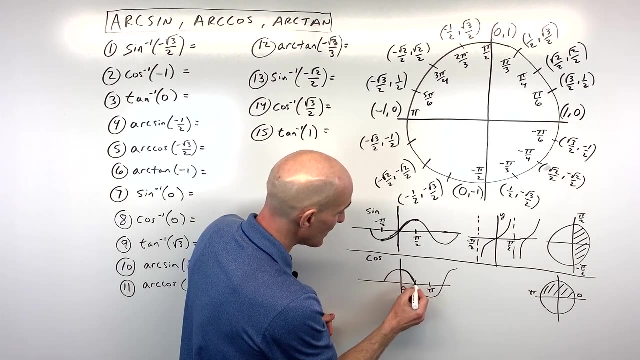 restrict it from negative pi over 2 to positive pi over 2 again. that puts us in the first and fourth quadrants over here to the right. now, when you look at cosine again, cosine repeats is failing that horizontal line test unless we restrict it from zero to pi. so we're just looking. 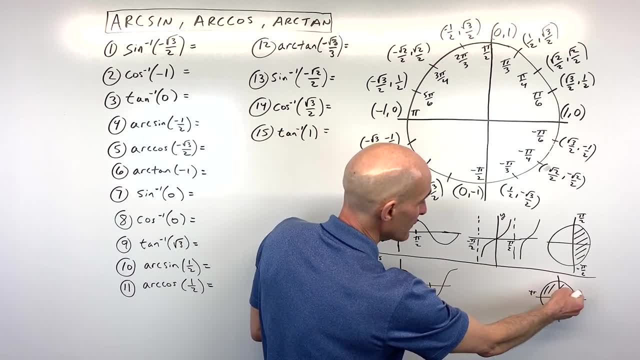 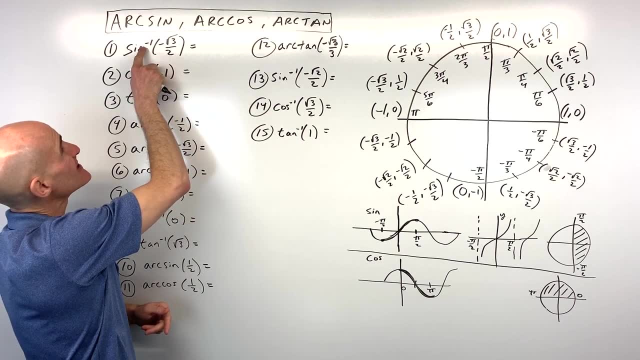 at this part of the graph right here. okay, and that's in the first and second quadrants. so let's go through some examples and then see if you can do these on your own. so if we want to find out what's the sine inverse of negative square root 3 over 2, 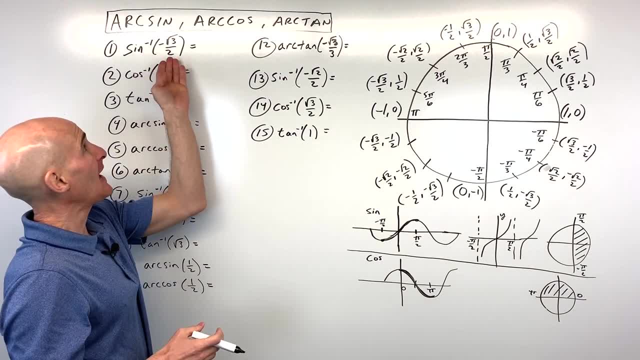 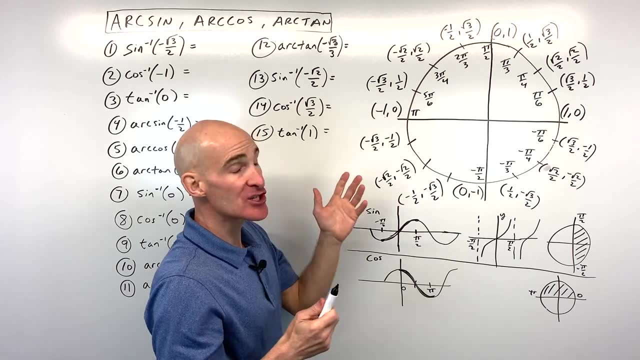 what that's really asking us is: sine of what angle equals negative square root 3 over 2? so what we can do is we can go to our unit circle- which i'm sure you probably memorize- if not, you can check out my mastering the unit circle video- and we say to ourselves: where is the sine negative root 3 over? 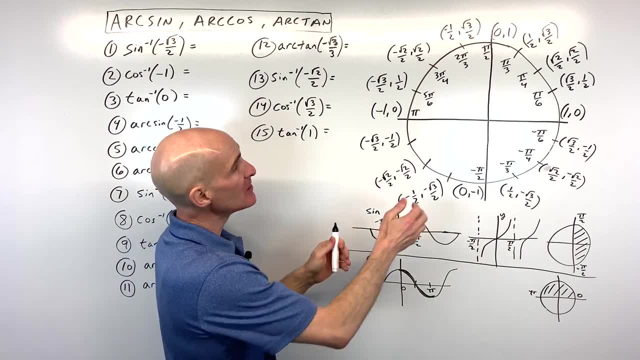 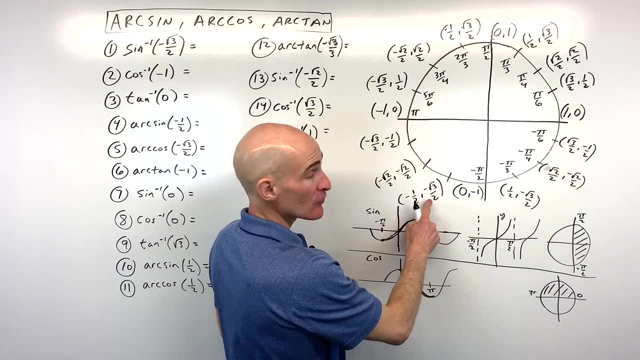 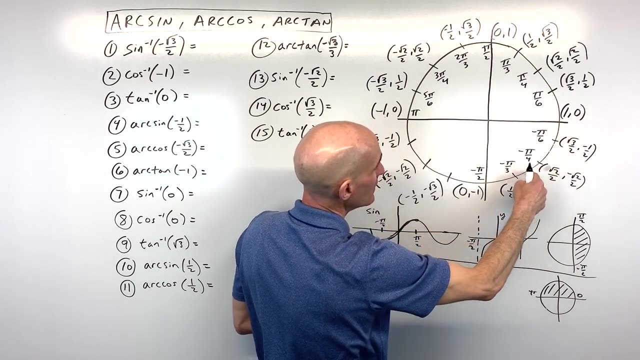 2. now remember, sine is the y coordinate on the unit circle. so we say: all right, well, i can know that the y is negative root 3 over 2. here it's also negative root 3 over 2, but remember we're just restricted from negative pi over 2 to positive pi over 2. so you can see i'm going. 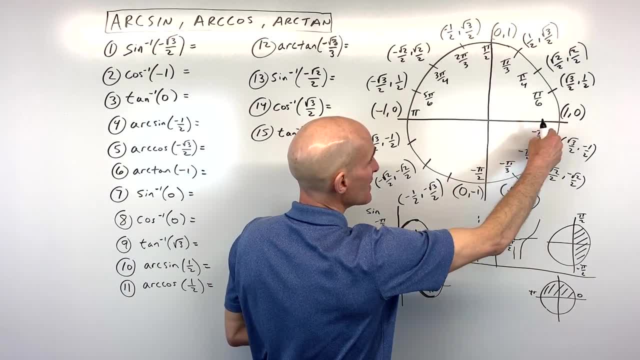 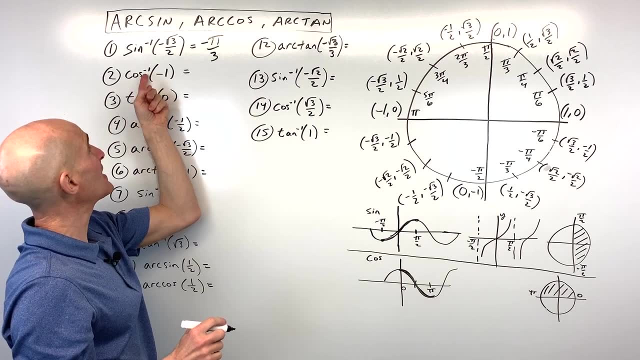 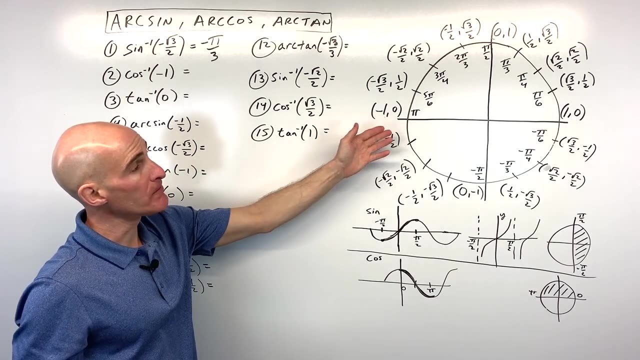 negative pi over 3. okay, you don't want to go all the way around like this, just make it a negative angle. so negative pi over 3 is our answer to that first one. for number two, what's the cosine inverse of negative 1? meaning, cosine of what angle equals negative 1.. now remember, on the unit circle, 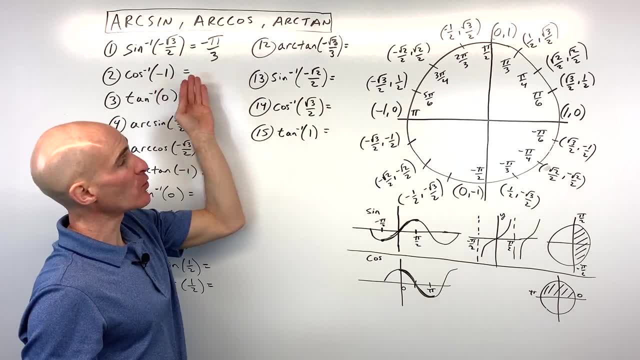 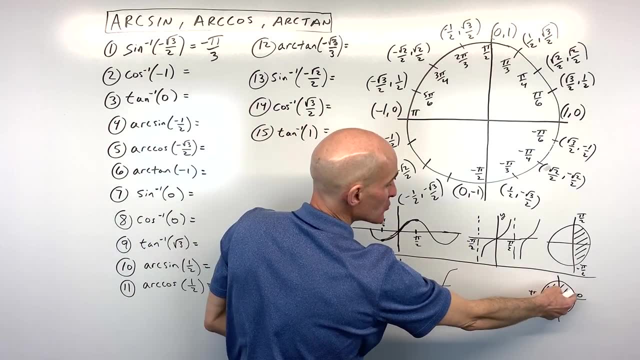 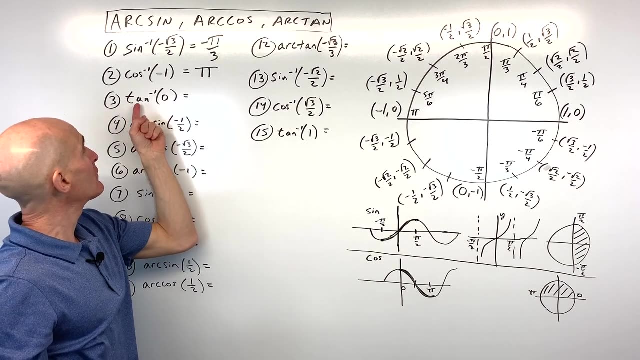 it's gonna be the x-coordinate, and remember where is the x-coordinate negative 1. that's going to be right here, at pi. and remember when we're solving for the cosine inverse restricted from 0 to pi. so you can see the answer here is going to be just pi. for number 3, what do you think for? 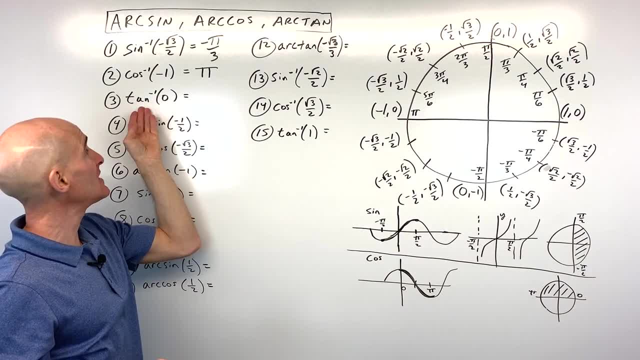 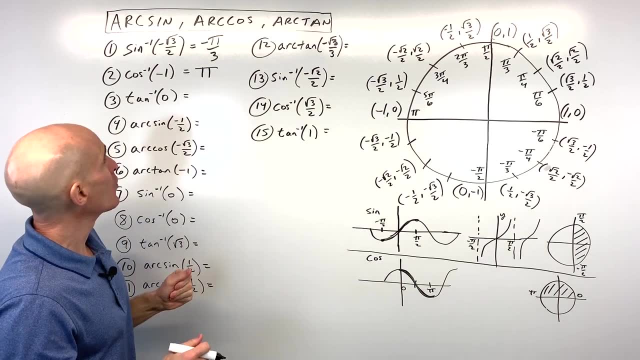 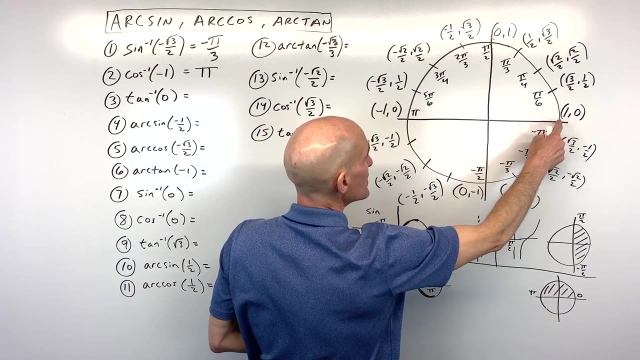 this one, the tangent inverse of zero. meaning the tangent of what angle equals 0.. remember, on the unit circle, tangent is the y divided by the x. okay, so where is the y coordinate divided by the coordinate zero? well, that would be here. zero over one is zero, okay, so this would be at zero radians. 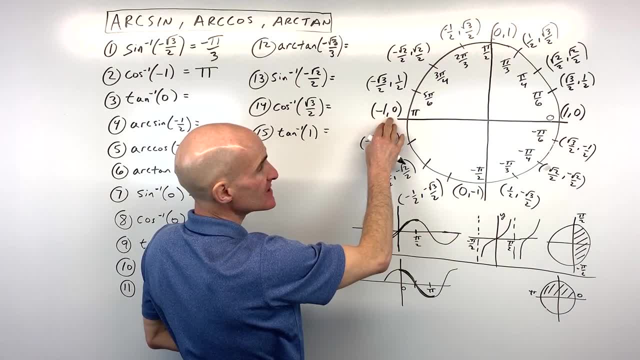 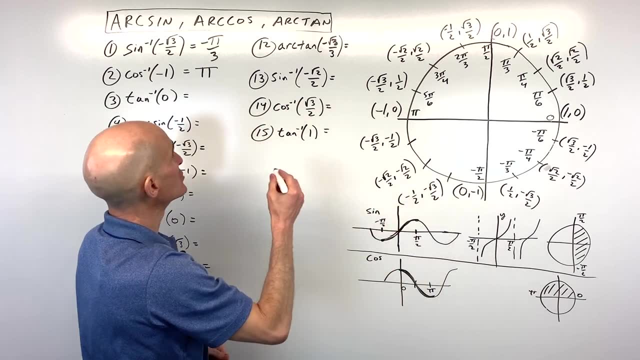 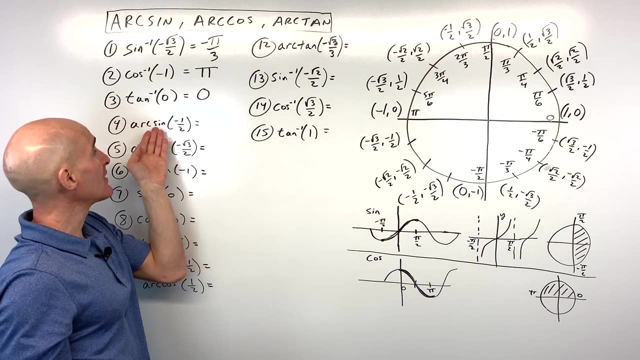 or it could be over here, but you can see this is not in the restricted domain. so for tangent inverse, we want to be from negative pi over two to positive pi over two, so it's just going to be zero radians. okay, for number four, what's the arc sine of negative one? half? now see. 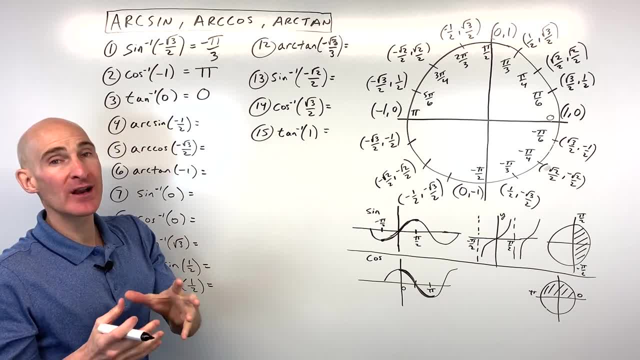 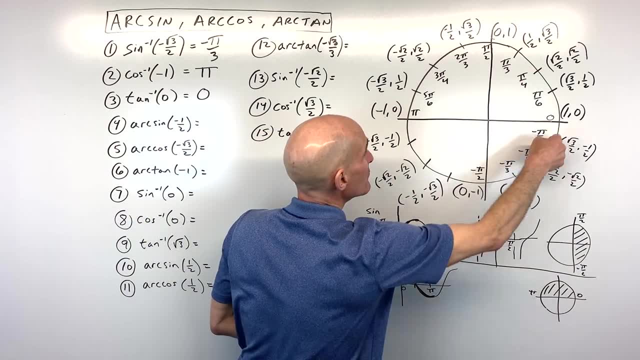 this arc, sine or sine inverse? it's just a different way of writing the same thing. this is just asking: a sine of what angle equals negative one half on this restricted domain, from negative pi over two to positive pi over two. well, remember, when we're talking about sine, we're looking for the y. 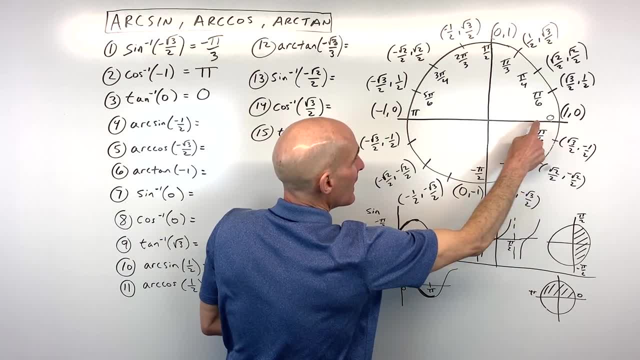 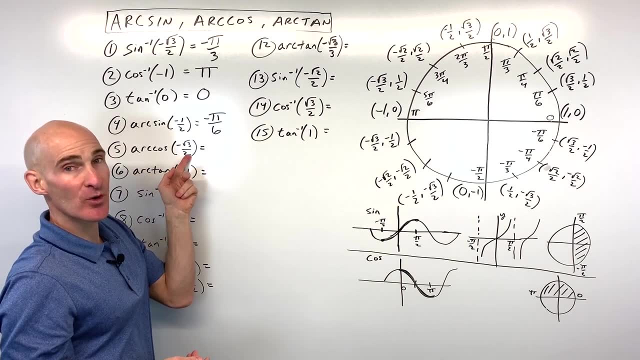 coordinates negative one half. that's going to be right here at negative pi over six. okay, let's look at number five. what's the arc cosine of negative square root three over two? meaning cosine of what angle equals negative root three over two? remember cosine. we're restricted. 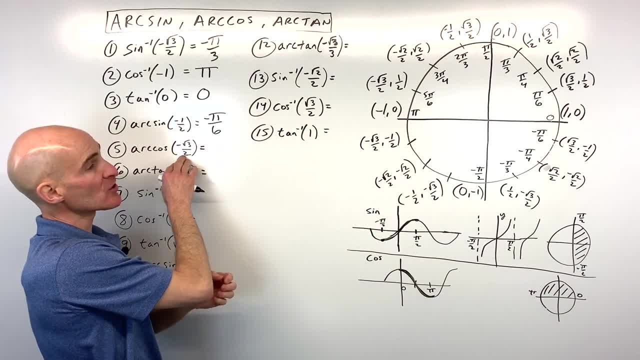 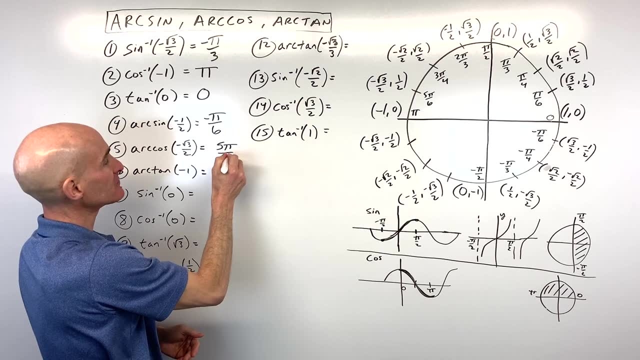 from zero to pi, that's in these first two quadrants. where does cosine equal negative root three over two? that's where the x coordinate is negative root three over two. that's going to be at five, pi over six. okay for number six, the arc tangent of negative. 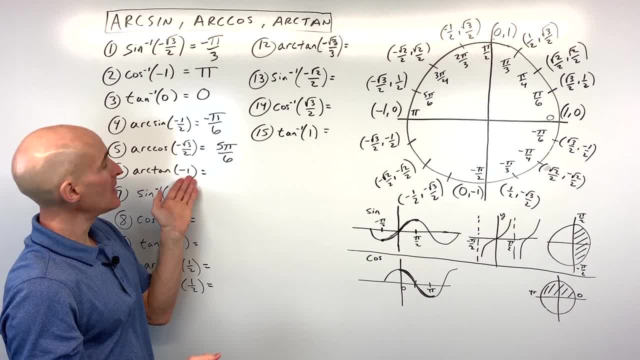 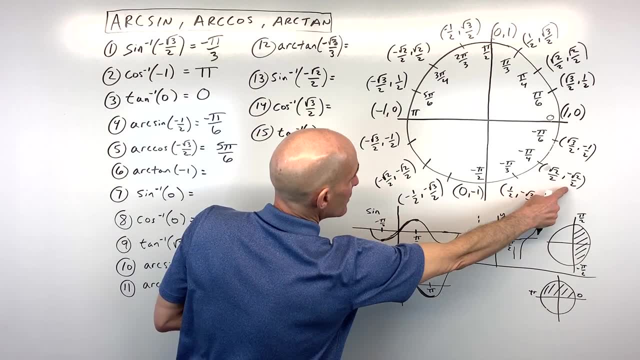 one. this is saying tangent of what angle equals negative one. and remember tangent on the unit circle is the y coordinate divided by the x coordinate. so you can see it's going to be negative one here, because anything divided by itself is one and negative divided by positive. 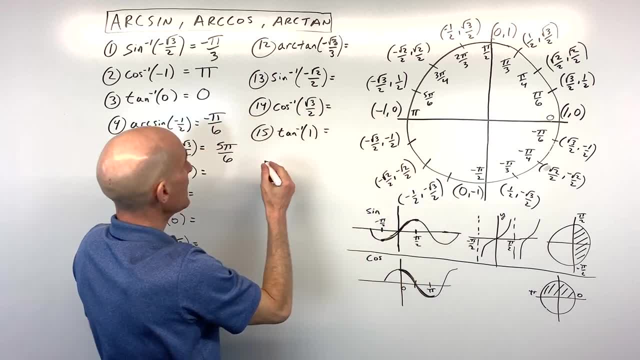 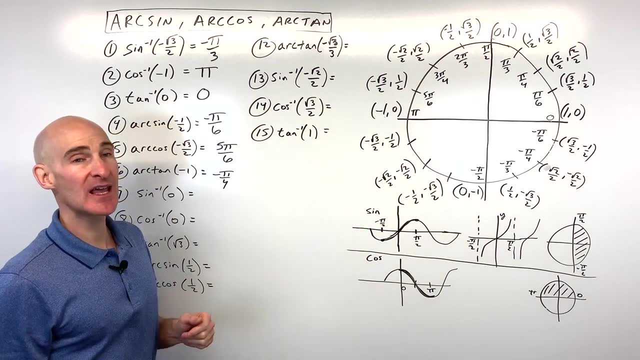 is a negative one. so this would be negative pi over four. okay, and that's going to be our answer because, remember, we're restricted from negative pi over two to positive pi over two, where we're doing the sine inverse or tangent inverse. what do you think for number seven? what's? 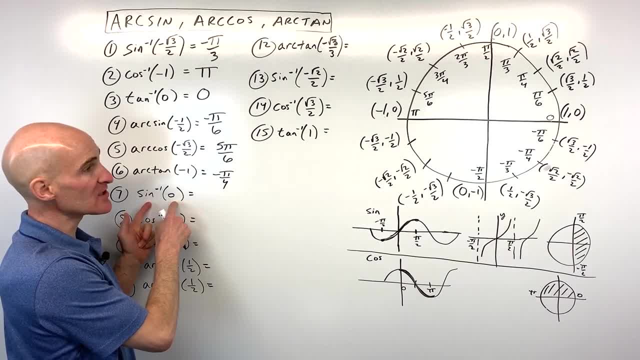 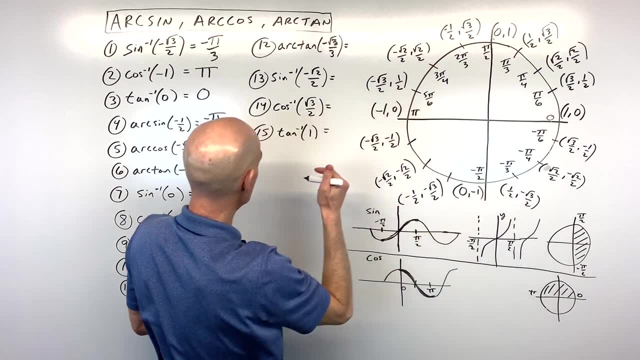 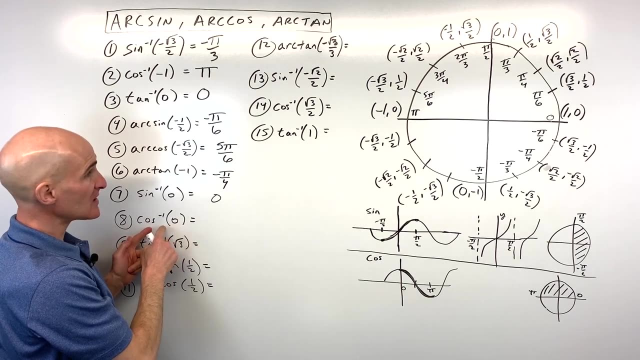 the sine inverse of zero. meaning, sine of what angle equals zero? well, sine, remember, is the y coordinate. you can see, the y coordinate is going to be zero right here, at zero radians. okay, how about number eight, the cosine inverse of zero. so, cosine of what angle equals zero? cosine on the 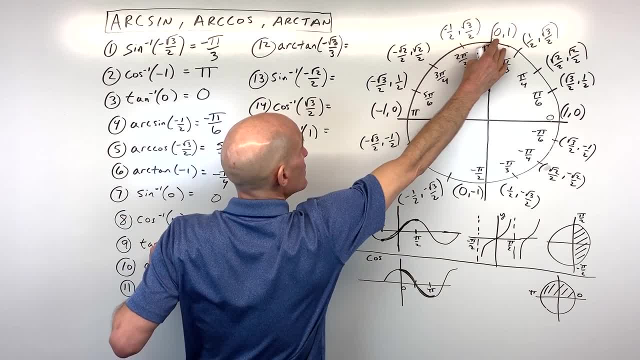 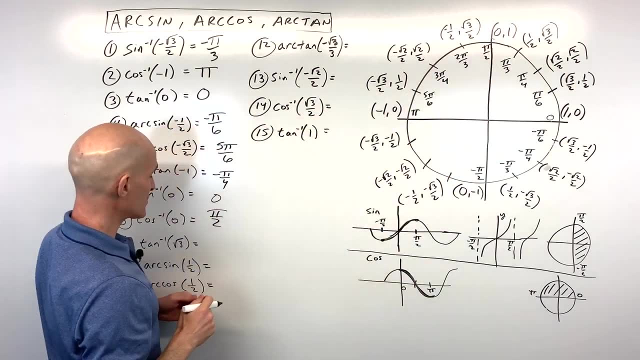 unit circle is the x coordinate. the x coordinate, zero, right here at pi over two. so that's going to be pi over two. and remember, with cosine inverse we're restricted from zero to pi. so it's just that. one solution for number nine, the tangent inverse of square root of three. okay, so this is saying: 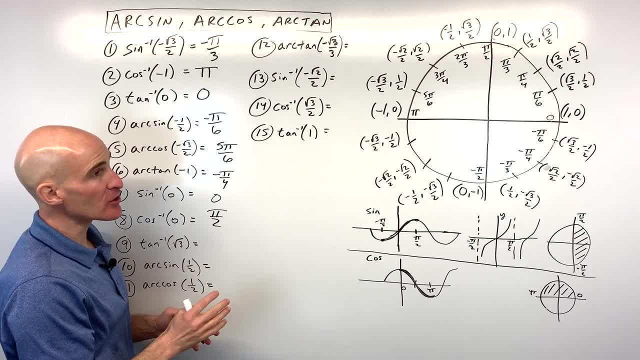 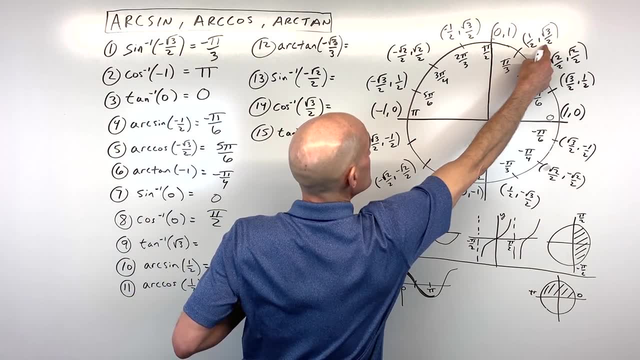 tangent of what angle equals square root of three. now remember, tangent is a little bit trickier: it's the y coordinate divided by the x coordinate. so here you can see, tangent is going to be root three at pi over three, because square root three over two divided by one half, gives you square root of. 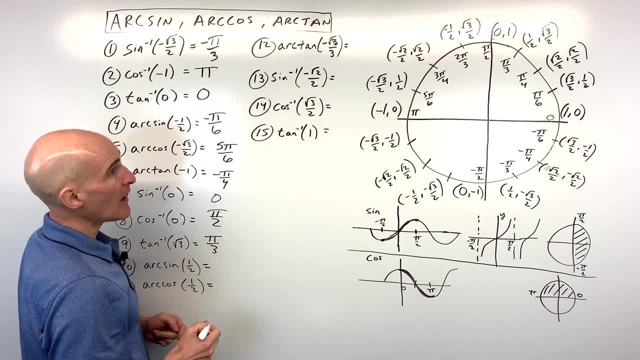 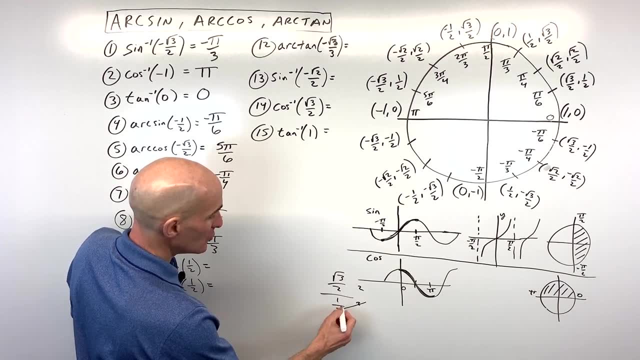 three. so what did we say? that was pi over three. now what you can do is: let's take square root of three over two divided by one half. see if you multiply the numerator and denominator by two. see how those twos cancel and you just get square root three over one. 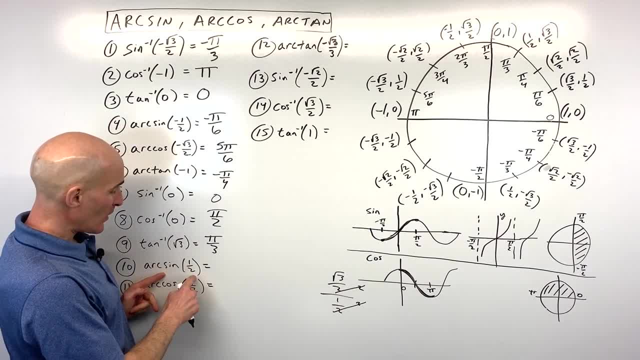 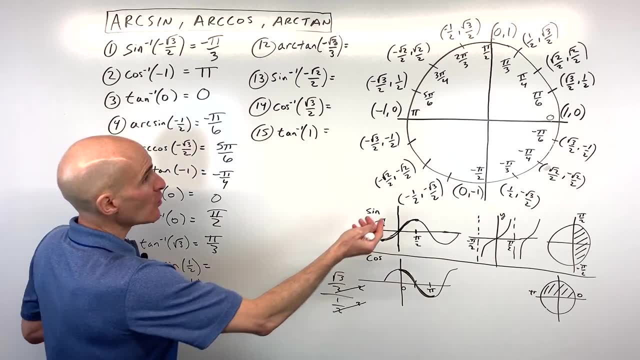 which is square root of three. for number ten, the arc sine of one half, this is saying sine of what angle equals one half. so remember, on the unit circles, sine is the y coordinate. where does the y coordinate equal one half? right here, at pi over six. and again, remember, we're restricted from here. 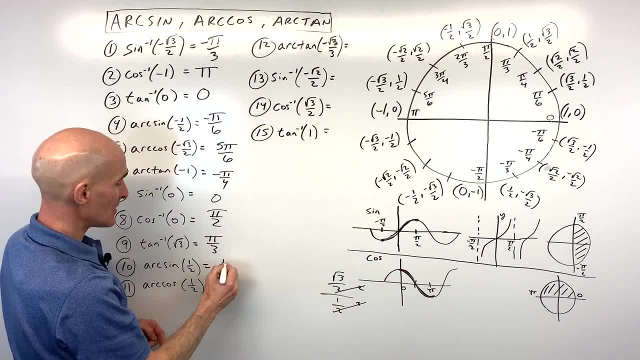 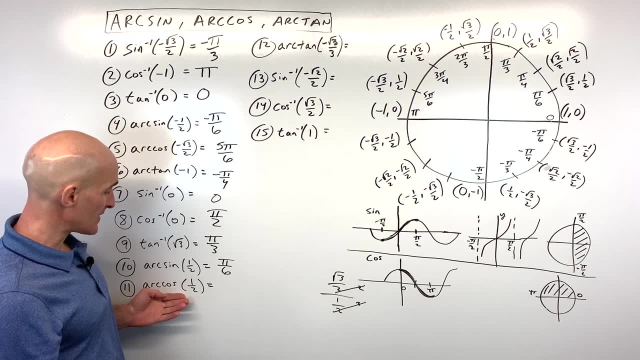 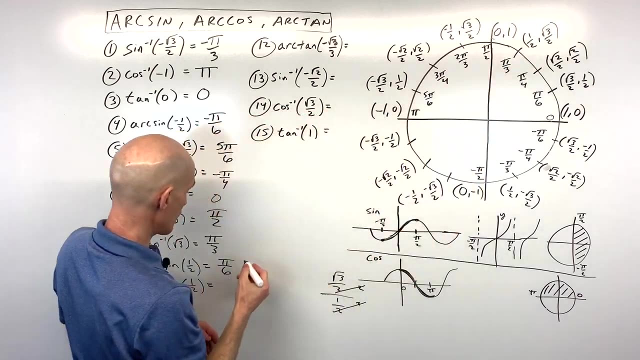 to here negative pi over two to positive pi over two, so that's pi over six. arc cosine of one, half cosine of what angle equals a half cosine? remember is the x coordinate. where is the x coordinate a half from zero to pi? that's going to be right here at pi over three. 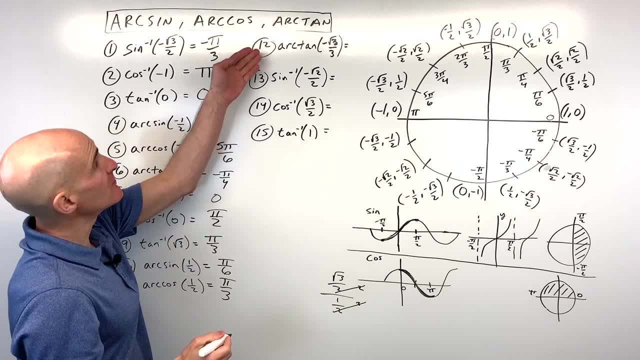 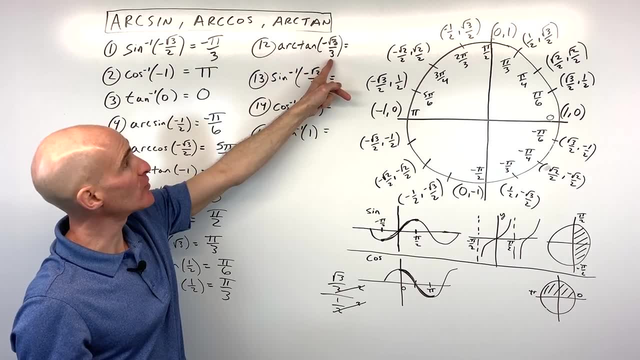 okay, number twelve, see if you can do this. one arc tangent of negative square root three over three. this is saying tangent of what angle equals negative root three over three? or where does the y coordinate divided by the x coordinate equal negative root three over three from negative pi. 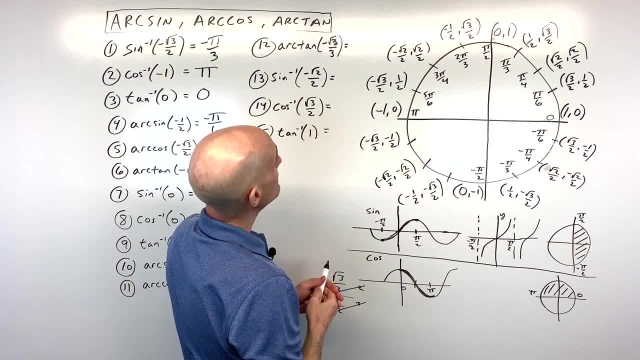 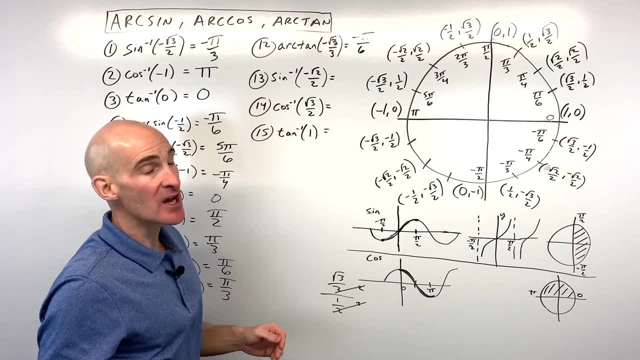 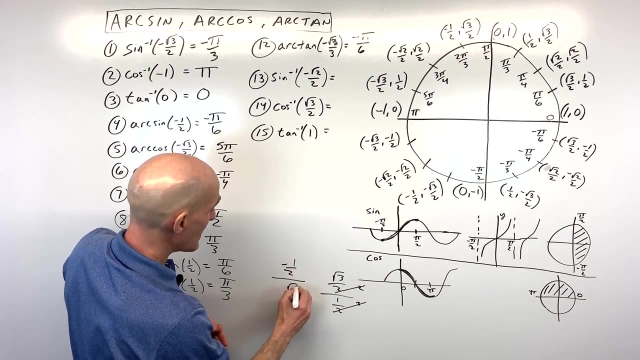 over two to positive pi over two. well, that's going to be right here. at negative pi over six. now, the tangent ones tend to be a little bit tougher. okay, because you have to divide the y by the x. but just to show you, here we have negative one half divided by positive square root. three over two again, if you. 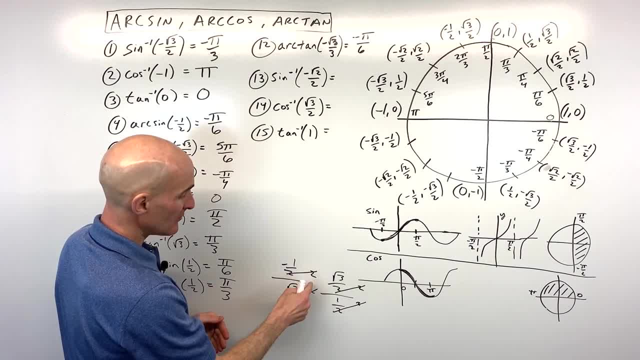 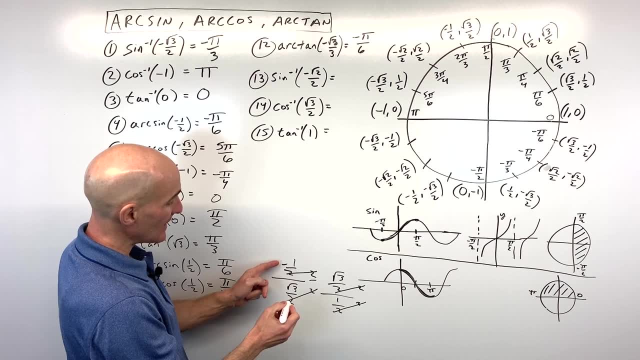 multiply the numerator and denominator by two, see how those cancel anything divided by itself. two divided by two is one, so that's not changing the value here of the fraction and we get negative one. and then, if you rationalize that by multiplying the numerator and denominator by square root of three, 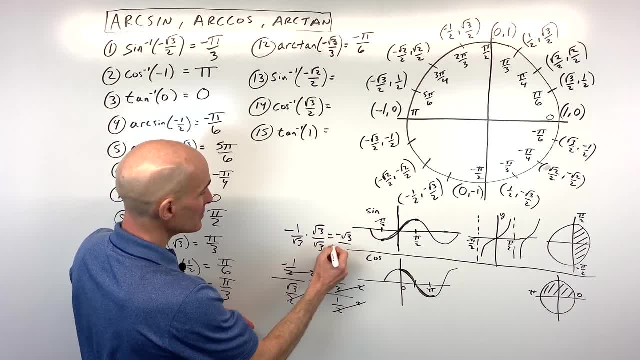 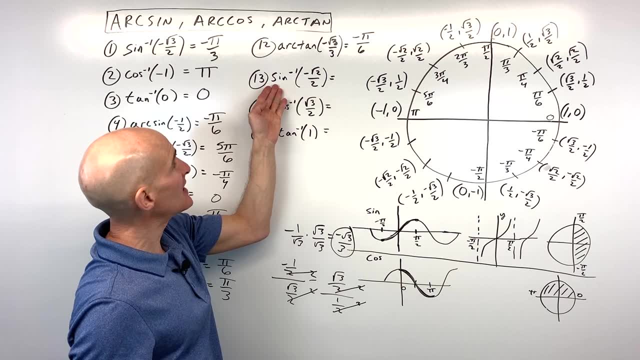 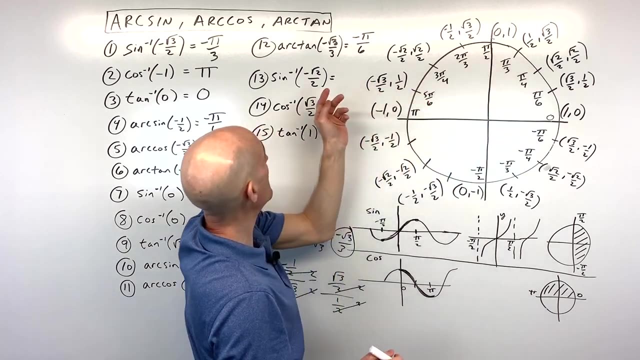 that gives you negative square root of three over square root of nine, which is three for number 13. what's the sine inverse of negative root two over two? well, this is saying we're. where is sine equal to negative root, two over two, from negative pi over two to positive pi over two? sine of the y. 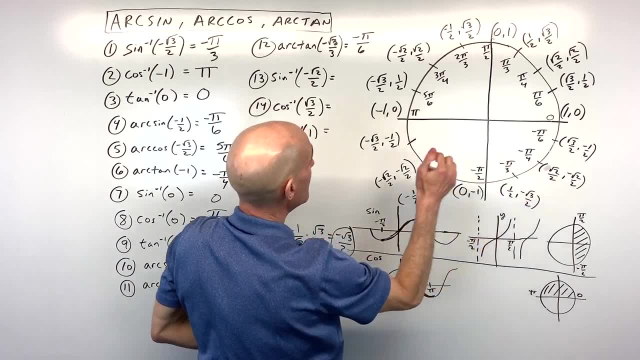 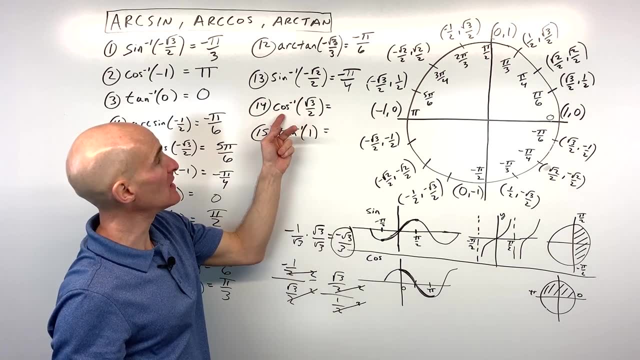 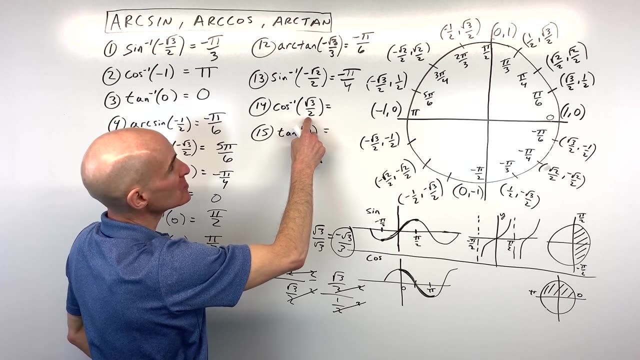 coordinate. so that's going to be right here at negative pi over four. okay, two more. so if you can do these last two, we've got cosine inverse of root 3 over 2, meaning cosine of what angle equal square root 3 over 2 from zero to pi. this is where the x coordinate is root 3 over 2.